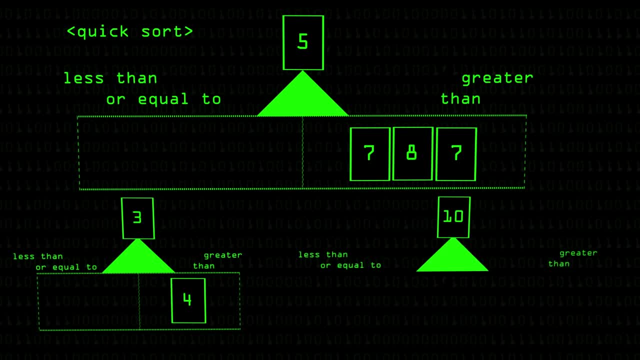 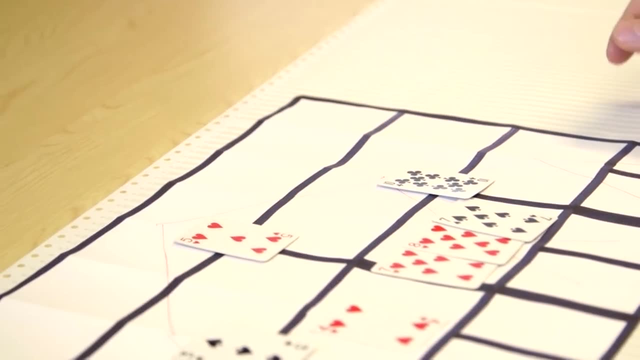 So with this one we take ten as the pivot, So everything less goes on the left, so it's actually all the elements, And then we keep breaking these down so we've got either one element or no elements in each list so that we know they're sorted. Okay, so we take seven. 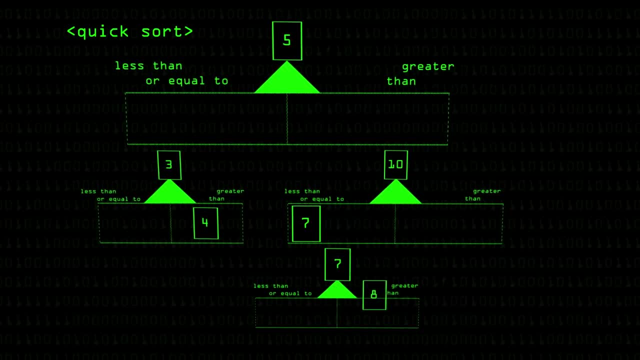 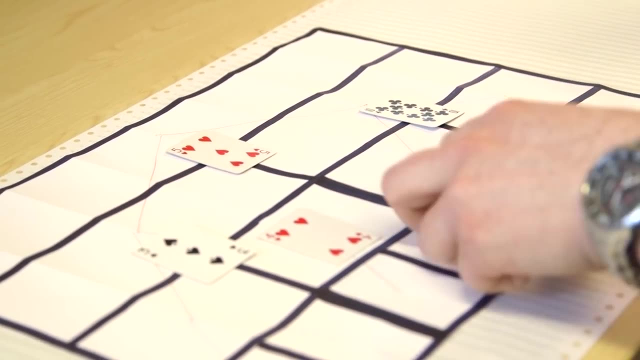 as the pivot, eight goes on the right and seven less than or equal goes on the left. So then we join all these lists back together, So start at the bottom. we take the pivot, everything on the left goes behind it, everything on the right goes on the left, And then we 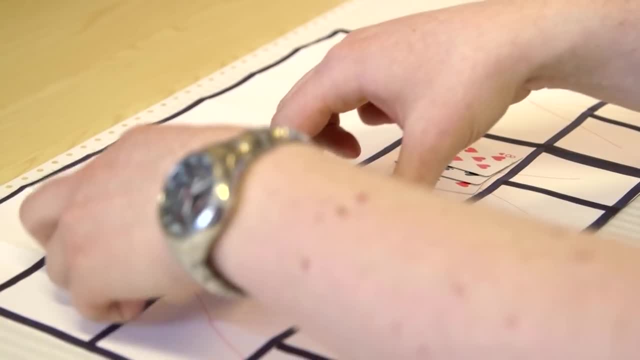 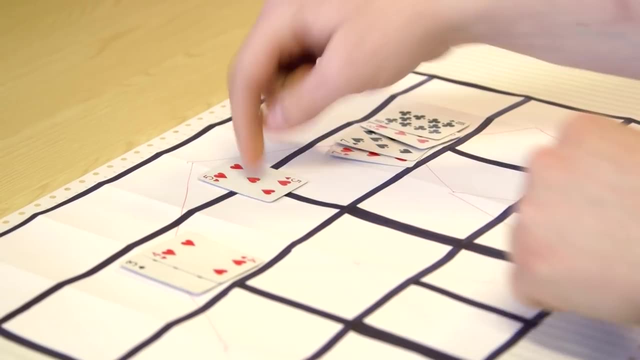 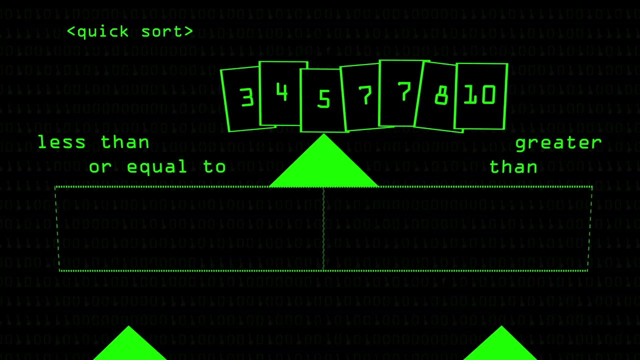 put four on top of it. Okay, so we've got the pivot here. put four on top of it. We've got ten here. everything on the left goes behind it, And then here we've got the pivot. so these go on its left and these go on its right. Okay, so now we've got one sorted list. 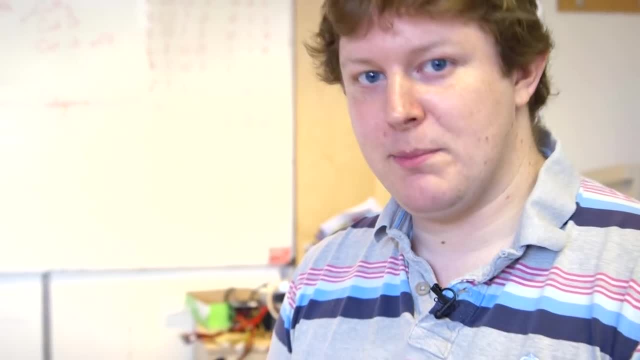 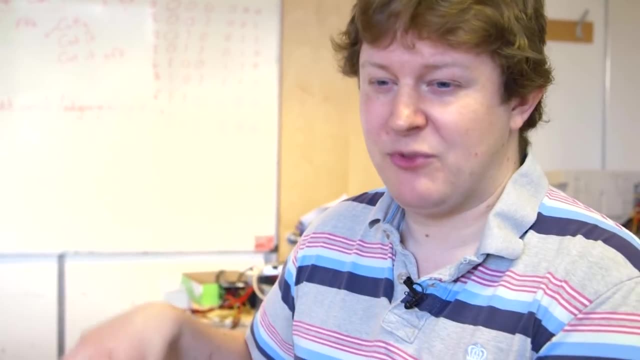 Now you do have to be careful about what you choose as the pivot. Usually, what they'll do is you'll either pick the first element or the last element, because it's just easier. Usually you want to be able to split the list into about two even parts, so really, 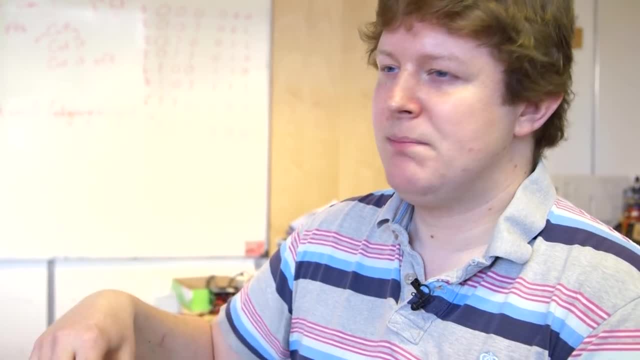 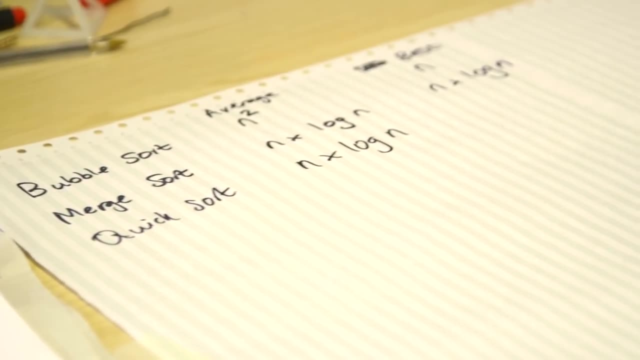 you want the pivot to be the middlemost number, But you don't know what that is at the start. So in the average case it's the same as the Merger Sort. We've got n times log n And in the best case it's still n log n. But in the worst case, well, let me show you Okay. 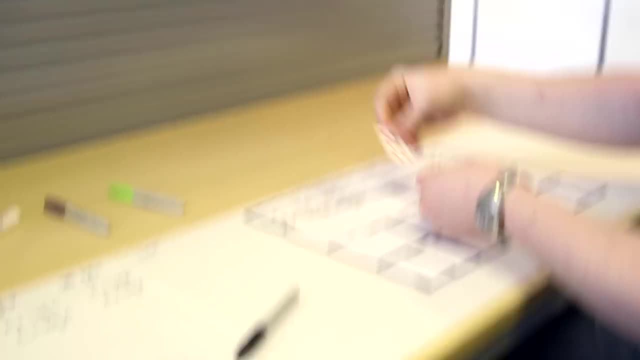 so let's say we've got a list that's already sorted, So I'll just take the cards we had before. If we always choose the pivot from the rightmost element, we've got ten, So ten's the pivot, And then we've got the pivot, And then we've got the pivot, So we've got the. 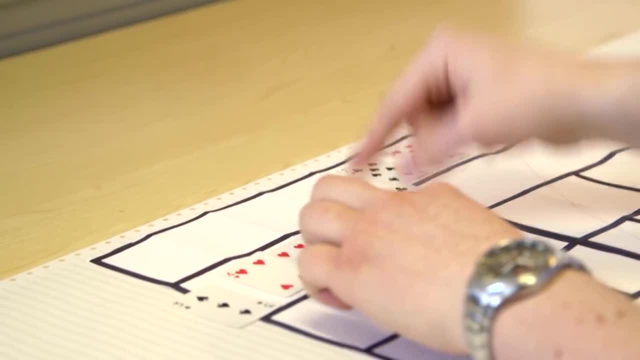 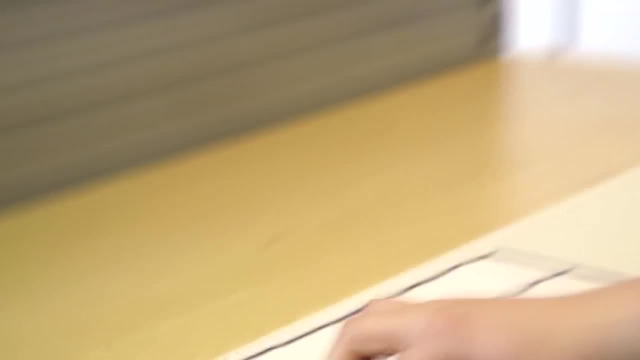 pivot. So all the elements less than it go on the left. So we've got all the elements, basically Okay. so then we pick eight as the next pivot. All the elements gone is left And we pick seven as the next. Then all the rest go on the left And we pick the next. 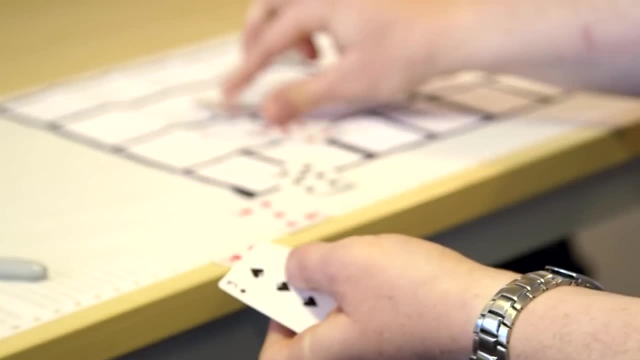 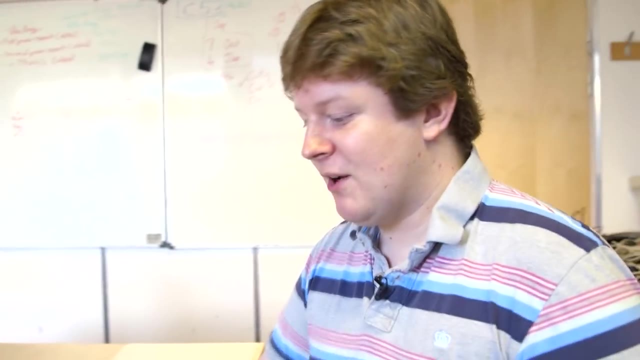 seven, And what you see is we end up with cards all the way down here, And then we've got to merge them back together, Okay, and actually that works out in the worst case, as n squared. So again it's the square of the input size.